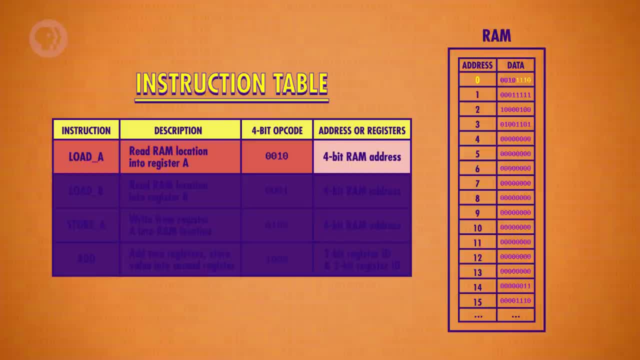 in those last 4 bits of the instruction and saves it into register A, In this case 1110, or 14 in decimal. So let's not think of this memory address 0 as 00101110, but rather as the instruction. 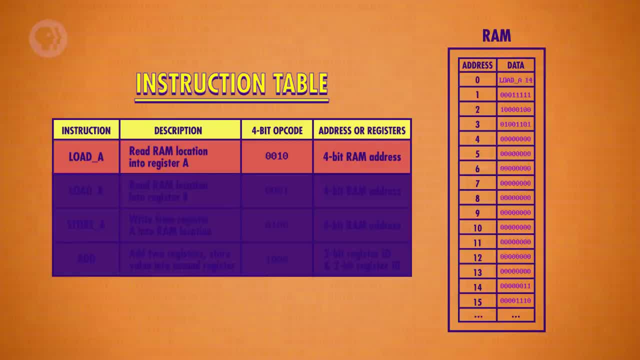 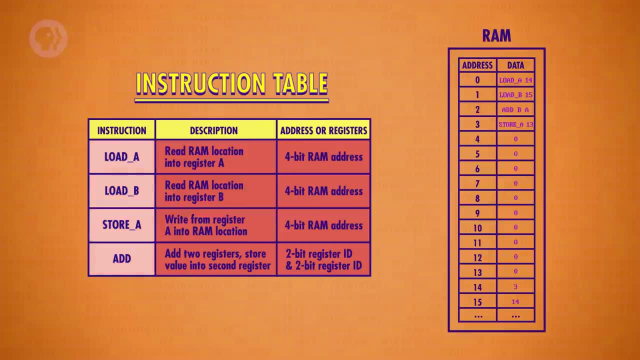 LOAD A14.. That's much easier to read and understand and for me to say- And we can do the same thing for the rest of the data in memory. In this case, our program is just 4 instructions long and we've put some numbers into memory. 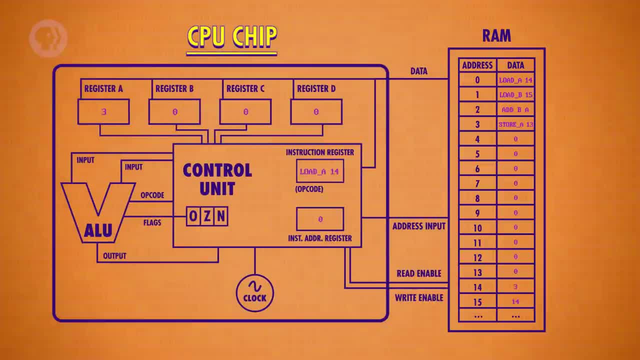 2, 3, and 14.. So now let's step through this program. First is LOAD A14,, which takes the value in address 14, which is the number 3, and stores it into register A. Then we have a LOAD B15 instruction, which takes the value in memory. 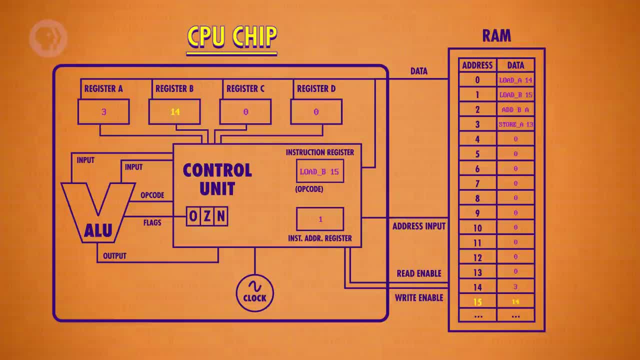 location 15,, which was the number 14, and saves it into register B. OK, easy enough, But now we have an ADD instruction. This tells the processor to use the ALU to add two registers together. In this case, B and A are specified. The ordering is important. 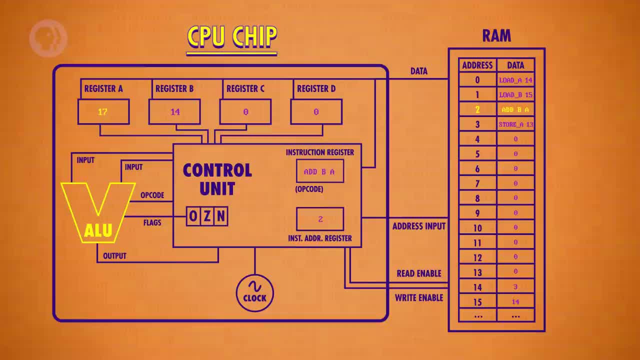 because the resulting sum is saved into the second register that's specified. So in this case the resulting sum is saved into register A. And finally, our last instruction is STORE A13, which instructs the CPU to write whatever value is in register A into memory location 13.. Yes, Our program adds two numbers together. 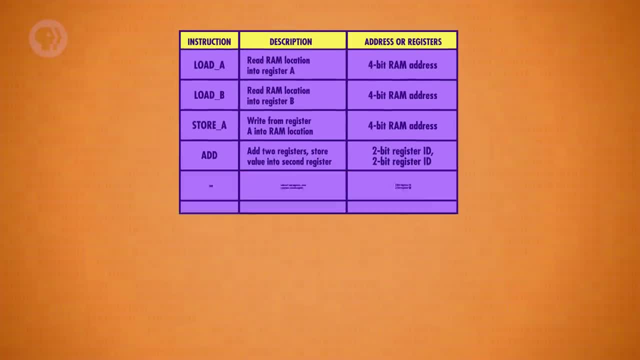 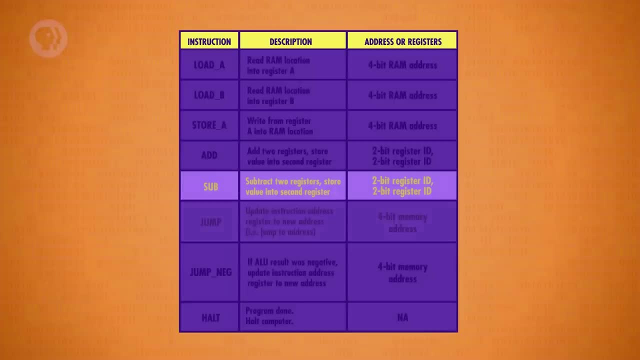 Exciting as it gets when we only have 4 instructions to play with, So let's add some more. Now we've got a SUBTRACT function which, like ADD, specifies two registers to operate on. We've also got a fancy new instruction called JUMP. As the name implies, this causes 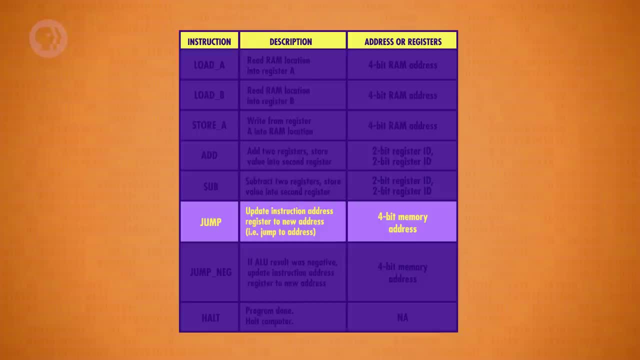 the program to jump to a new location. This is useful if you want to change the order or skip some instructions. For example, a JUMP 0 would cause the program to go back to the beginning At a low level. this is done by writing the value specified in the 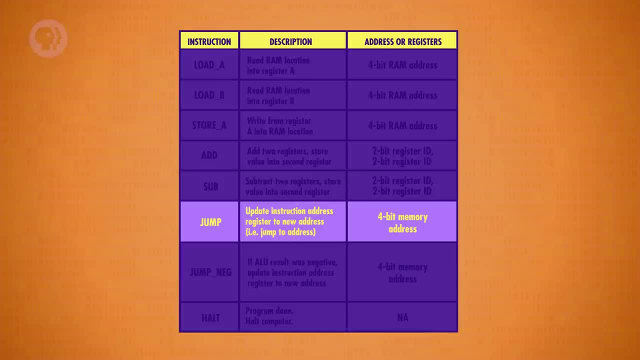 last 4 bits into the instruction address register, overwriting the current value. We've also added a special version of JUMP called JUMP NEGATIVE. This only jumps the program if the ALU's negative flag is set to true, As we talked about in episode 5,. 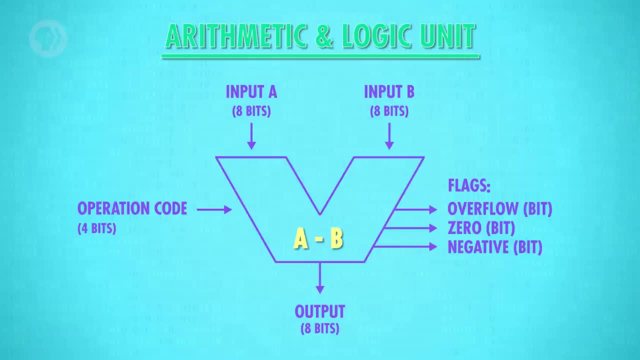 the negative flag is only set when the result of an arithmetic operation is negative. If the result was 0 or positive, the negative flag would not be set, so the JUMP NEGATIVE wouldn't jump anywhere and the CPU will just continue on to the next instruction. 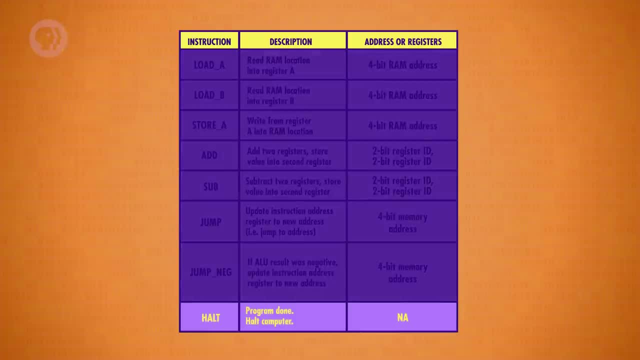 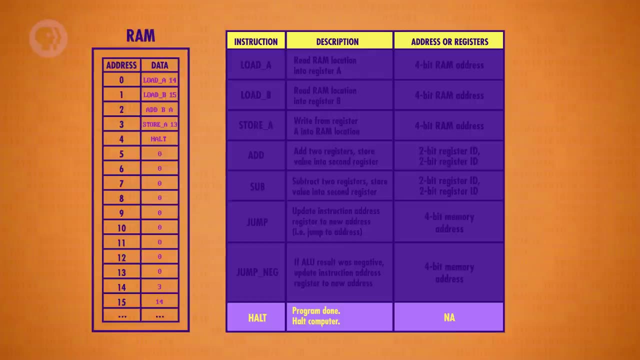 And finally, computers need to be told when to stop processing, so we need a HALT instruction. Our previous program really should have looked like this to be correct. Otherwise the CPU would have just continued on after the store instruction, processing all those 0s. But there is no instruction with an opcode of 0, and so the computer would. 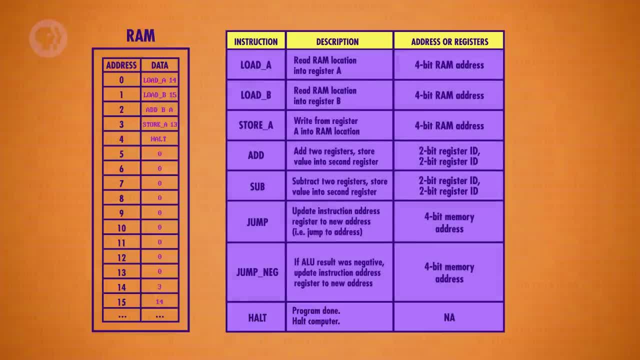 have just crashed. It's important to point out here that we're storing both instructions and data in the same memory. There is no difference. fundamentally, it's all just binary numbers. So the HALT instruction is really important because it allows us to separate the two. 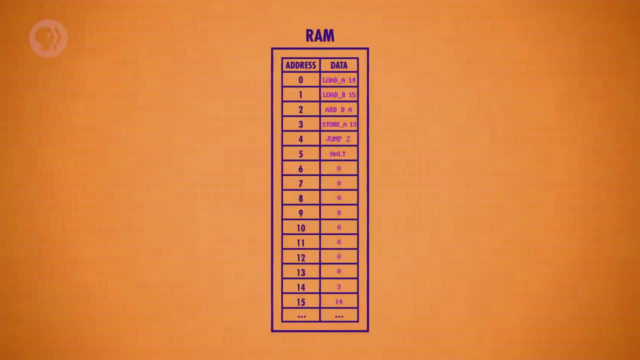 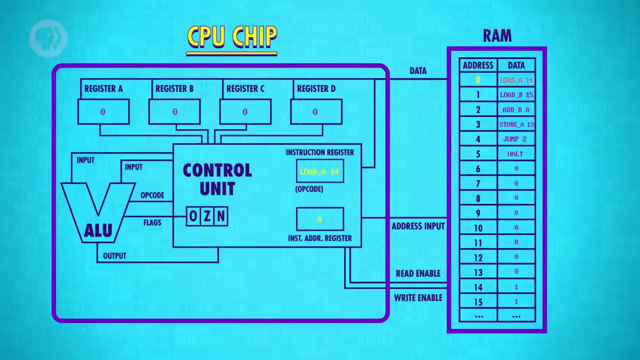 OK, so let's make our program a bit more interesting by adding a JUMP. We'll also modify our two starting values in memory to 1 and 1.. Let's step through this program as fast as our CPU would. First, LOAD A 14 loads the value 1 into register A. Next, LOAD B 15 loads the value 1 into. 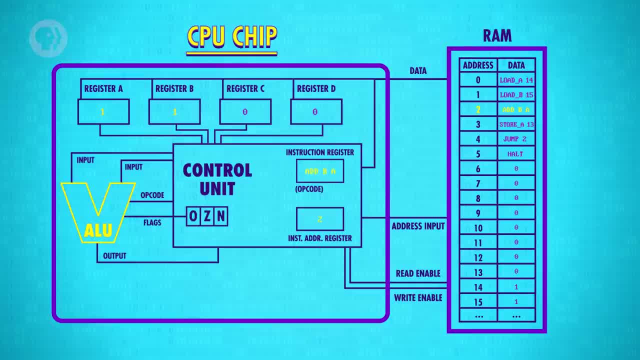 register B. As before, we add registers B and A together with the sum going into register A. 1 plus 1 equals 2, so now register A has the value 2 in it, stored in binary, of course. Then the STORE instruction saves that into memory location 13.. 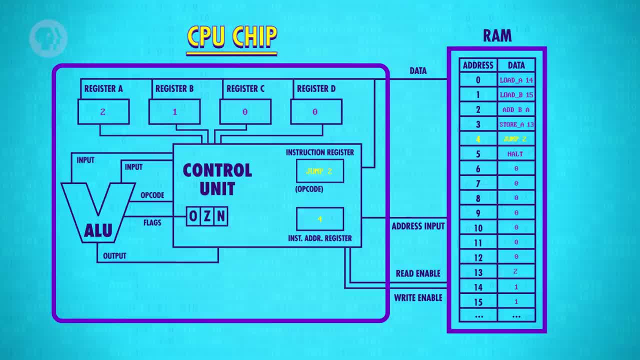 Now we hit a JUMP 2 instruction. This causes the processor to overwrite the value in the instruction address register, which is currently 4, with the new value 2.0.. Let's see what we can do On the processor's next fetch cycle. we don't fetch HALT. Instead we fetch the instruction. 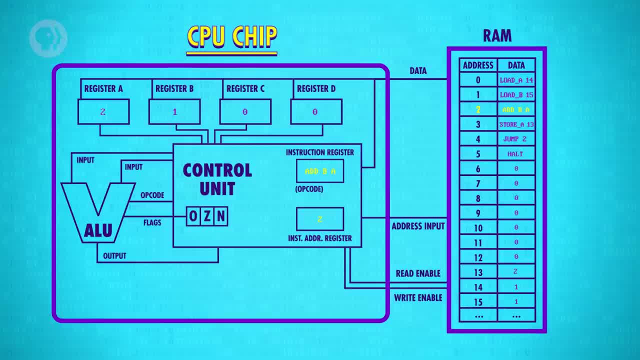 of memory location 2,, which is ADD BA. We've jumped. Register A contains the value 2, and register B contains the value 1, so 1 plus 2 equals 3.. So now register A has the value 3.. We store that into memory And we've hit the JUMP. 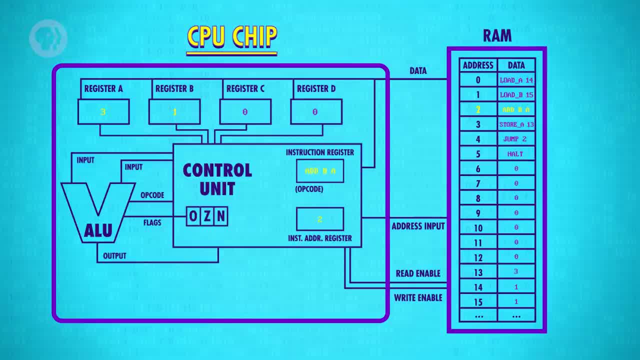 again back to ADD BA. 1 plus 3 equals 4, so now register A has the value 4.. See what's happening here. Every loop we're adding 1.. It's counting up, Cool, But notice there's no way to edit this. 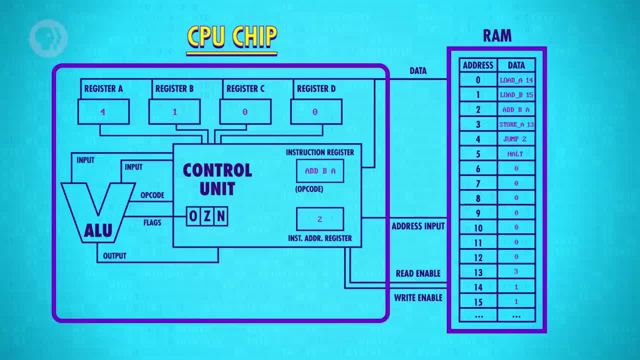 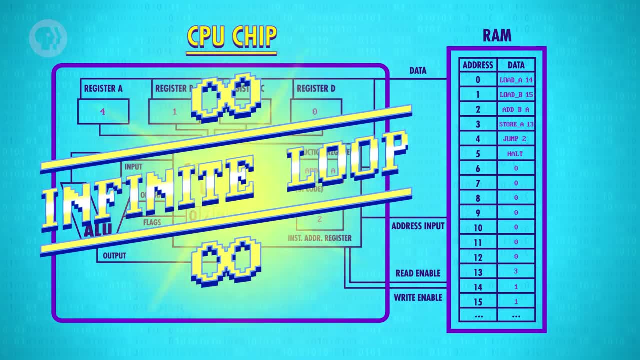 We're never, ever going to hit that HALT instruction, because we're always going to hit that JUMP. This is called an infinite loop, a program that runs forever. To break the loop, we need a conditional JUMP, a jump that only happens if a certain condition. 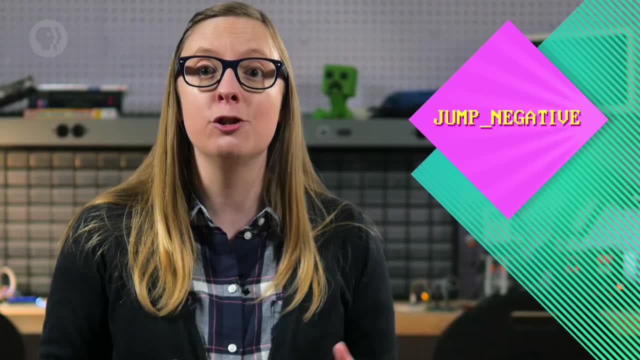 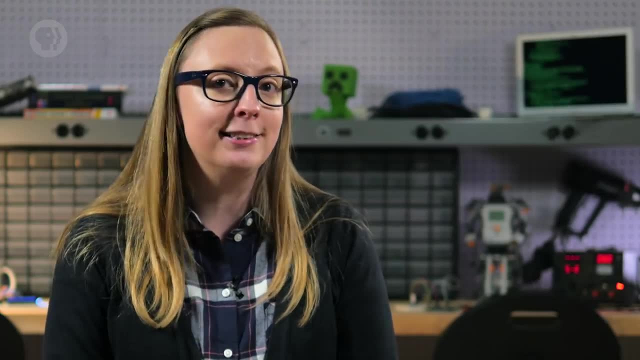 is met. Our JUMP negative is one example of a conditional jump, but computers have other types too, like JUMP IF equal and JUMP IF greater. So let's make our code a little fancier and step through it Just like before the program starts by loading values in the program. 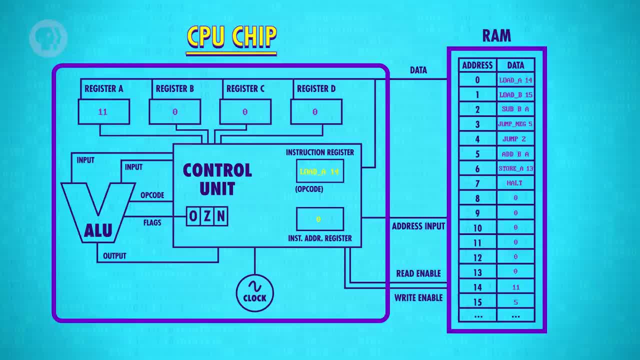 We're loading values from memory into registers A and B. In this example, the number 11 gets loaded into register A and 5 gets loaded into register B. Now we subtract register B from register A, That's 11 minus 5, which is 6, and so 6. 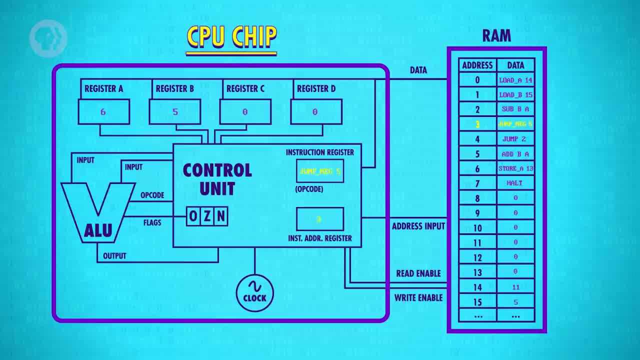 gets saved into register A. Now we hit our JUMP negative. The last ALU result was 6, that's a positive number, so the negative flag is false. That means the processor does not jump. so we continue on to the next instruction, which is JUMP 2.. No conditional on this one, so we jump. 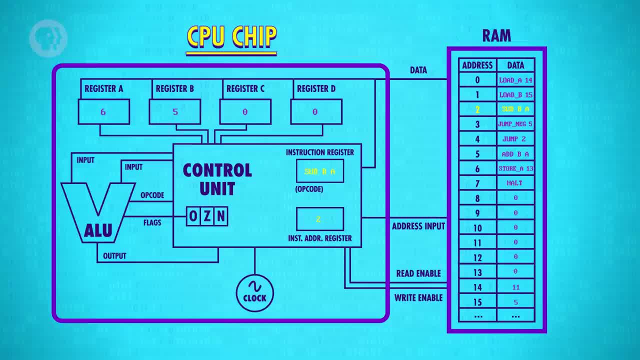 to instruction 2, no matter what. OK. so we're back at our subtract. register B from register A: 6 minus 5 equals 1, so 1 gets saved into register A. Next instruction: We're back again at our JUMP. negative 1 is also a positive number. 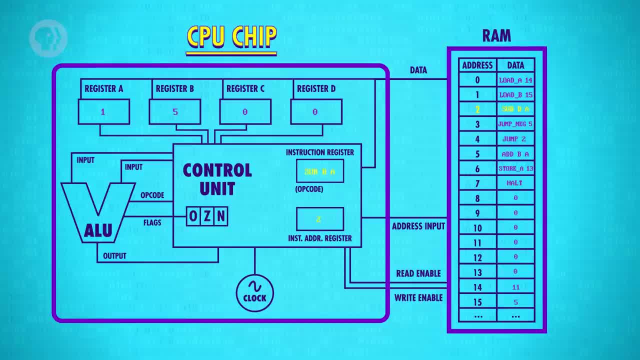 so the CPU continues on to the JUMP 2, looping back around again to the subtract instruction. This time is different, though: 1 minus 5 is negative 4, and so the ALU sets its negative flag to true for the first time. 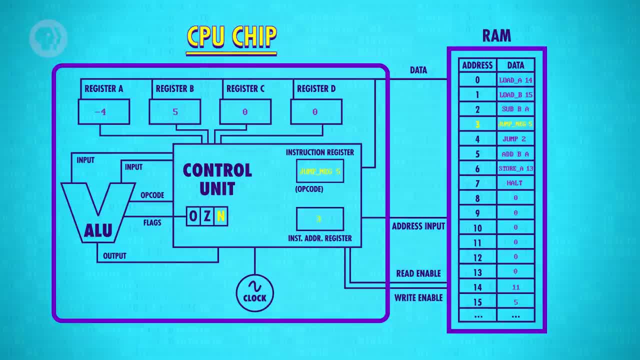 Now, when we advance to the next instruction, JUMP negative 5, the CPU executes the jump to memory location 5.. We're out of the infinite loop. Now we have an ADD B to A Negative. 4 plus 5 is positive. 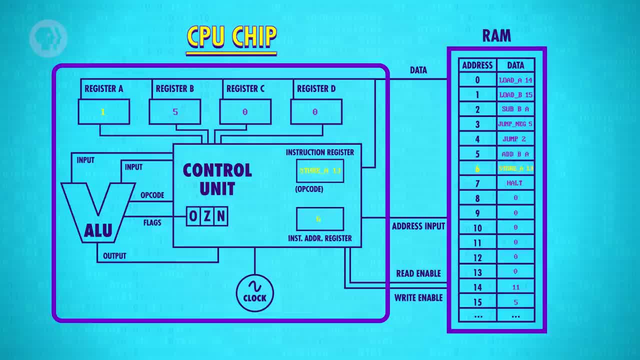 1, and we save that into register A. Next, we have a STORE instruction that saves register A into memory address 13.. Lastly, we hit our HALT instruction and the computer rests. So even though this program is only 7 instructions long, the CPU ended up executing 13 instructions. 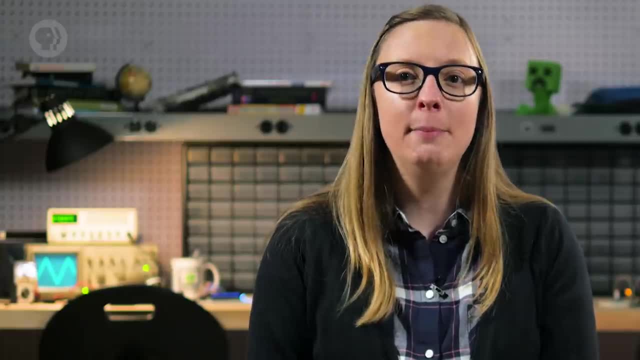 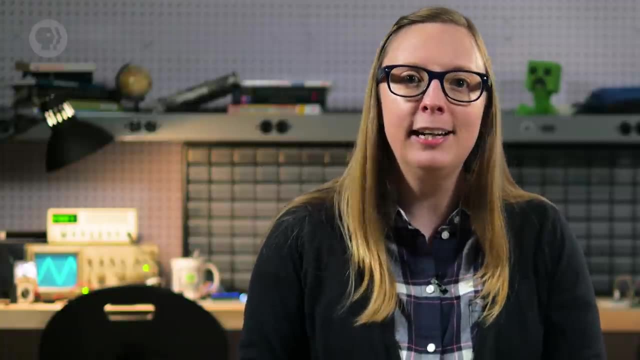 and that's because it looped twice internally. This code calculated the remainder if we divide 5 into 11, which is 1.. With a few extra lines of code, we could also keep track of how many loops we did The count. 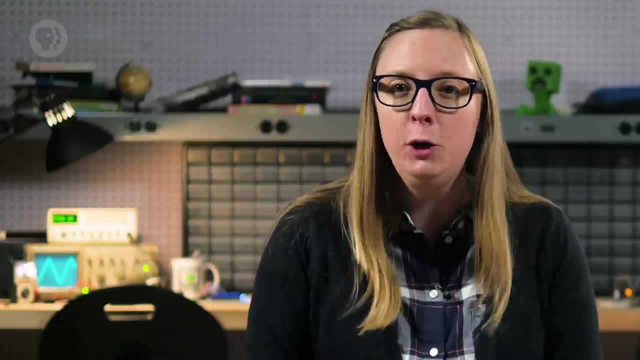 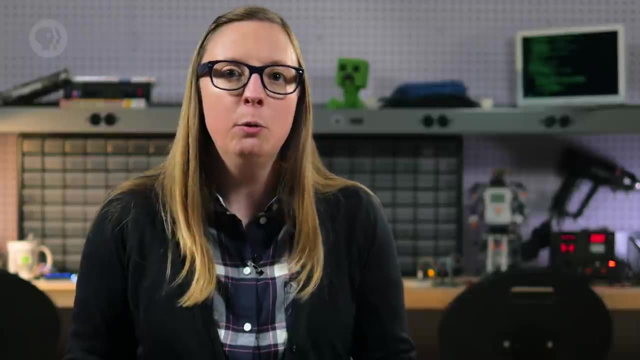 of which would be how many times 5 went into 11.. We did two loops, so that means 5 goes into 11 two times, with a remainder of 1.. And of course this code could work for any two numbers which we can just change in memory. 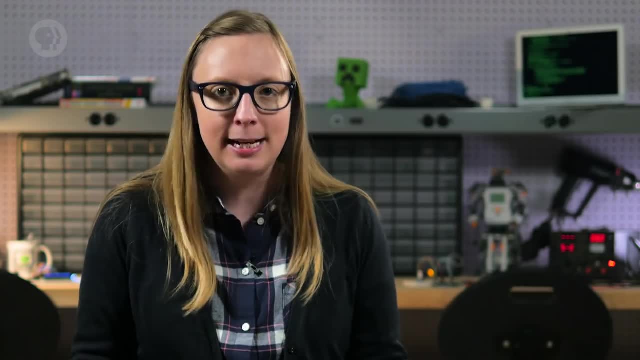 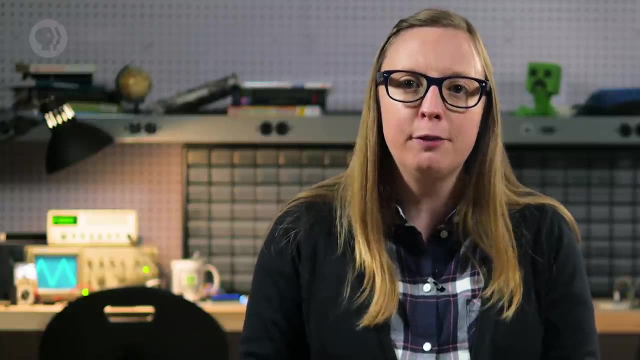 to whatever we want: 7 and 81,, 18 and 54, it doesn't matter. That's the power of software. Software also allowed us to do something our hardware could not Remember. our ALU didn't have the functionality to divide two numbers. Instead, it's the power of software that 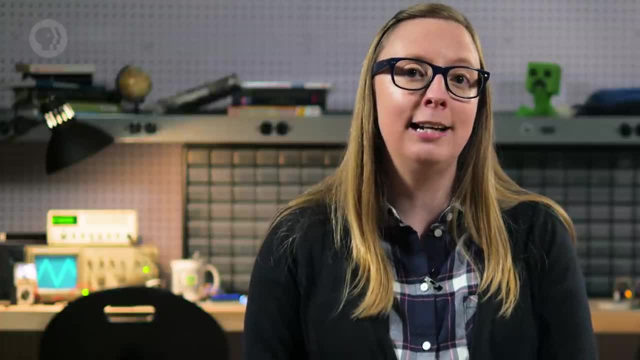 allows us to do something. our hardware could not. Remember: our ALU didn't have the functionality to divide two numbers. Instead, it's the power of software that allows us to do something our hardware could not. Instead, it's the power of software that allows us to do something our hardware could not. Instead, it's the 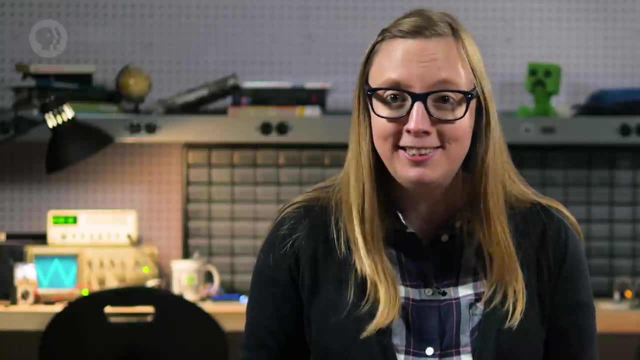 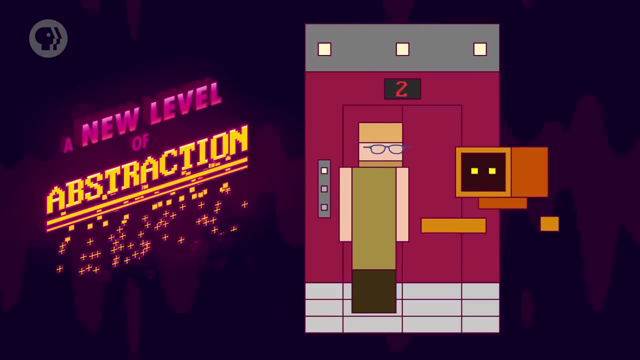 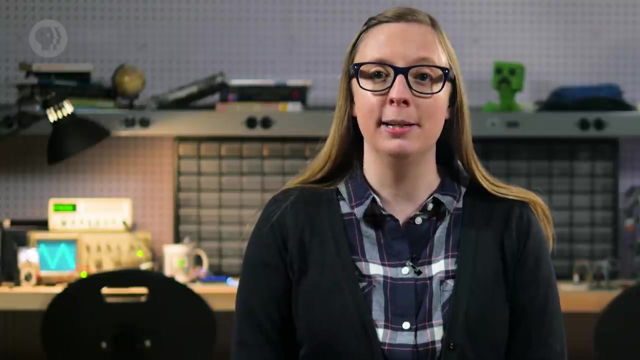 power of software that allows us to divide two numbers, which gives us the functionality we want. Then another program used it to divide two numbers was the divide program, and you know what that means: New levels of abstraction. So our hypothetical CPU is very basic. All of its instructions are 8 bits long, with 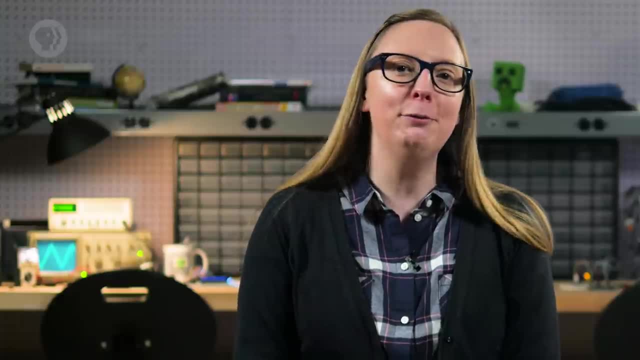 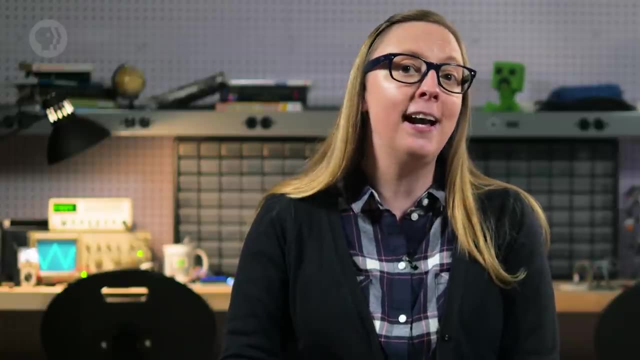 the opcode occupying only the first 4 bits. So even if we used every combination of 4 bits, our CPU would only be able to support a maximum of 16 different instructions. different instructions On top of that, several of our instructions use the last 4 bits to specify a memory location. 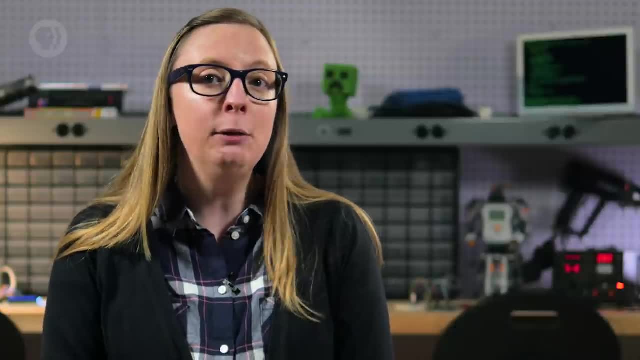 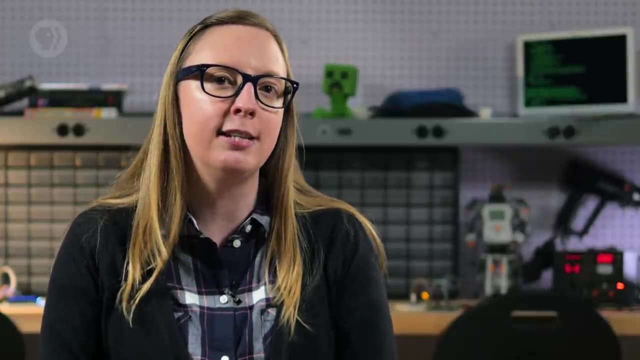 But again, 4 bits can only encode 16 different values, meaning we can address a maximum of 16 memory locations. That's not a lot to work with. For example, we couldn't even jump to location 17, because we literally can't fit the number. 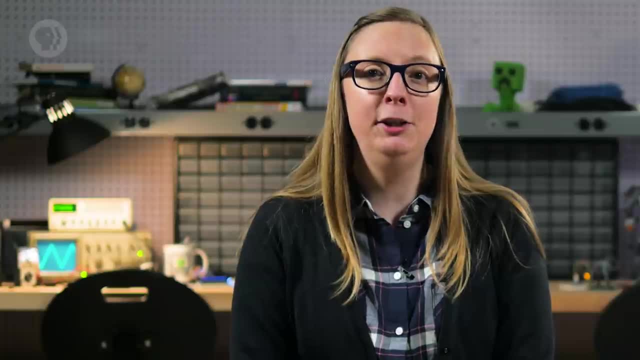 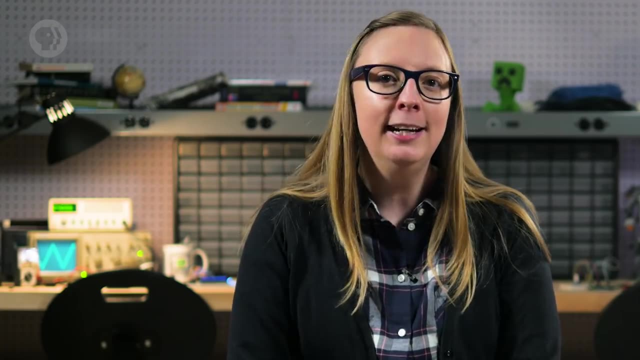 17 into 4 bits. For this reason, real modern CPUs use two strategies. The most straightforward approach is just to have bigger instructions with more bits, like 32 or 64 bits. This is called the instruction length, unsurprisingly. 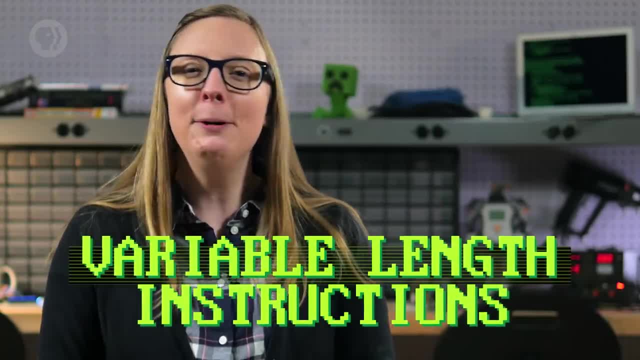 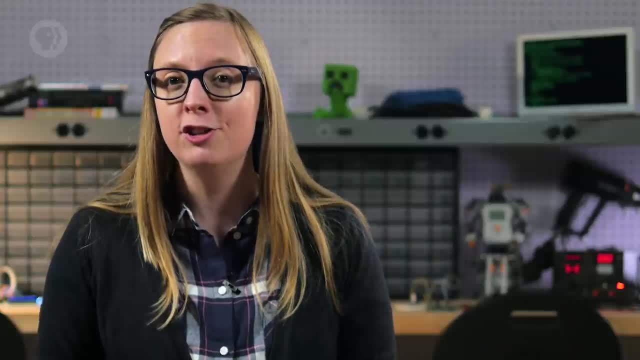 The second approach is to use variable length instructions. For example, imagine a CPU that uses 8-bit opcodes. When the CPU sees an instruction that needs no extra values, like the HALT instruction, it can just execute it immediately. However, if it sees something like a JUMP instruction, it knows it must also fetch the 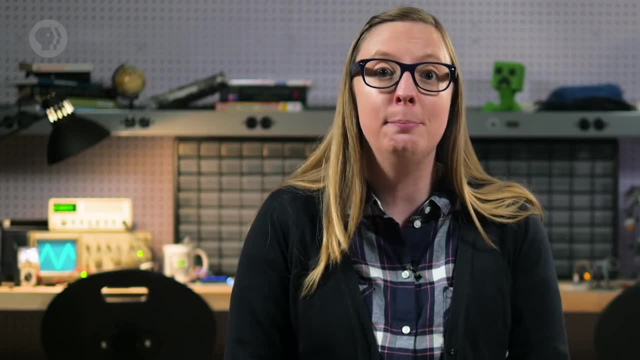 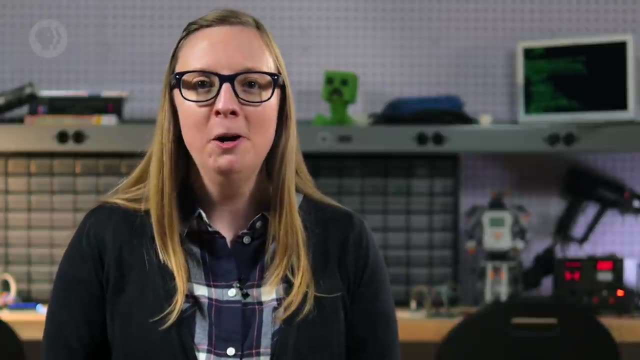 address to jump to, which is saved immediately behind the JUMP instruction in memory. This is called, logically enough, an immediate value. In such processes, instructions can be any number of bytes long, which makes the fetch cycle of the CPU a tad. 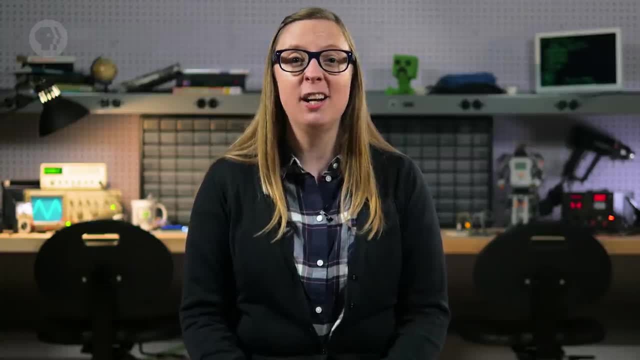 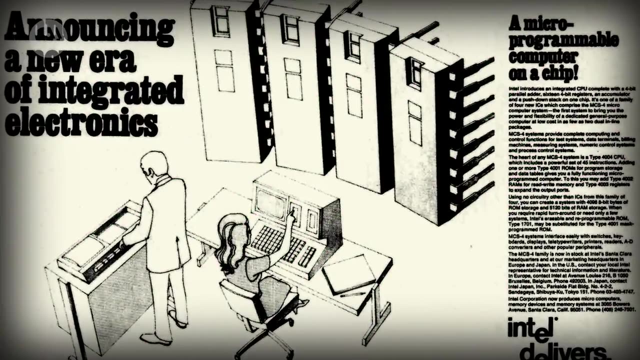 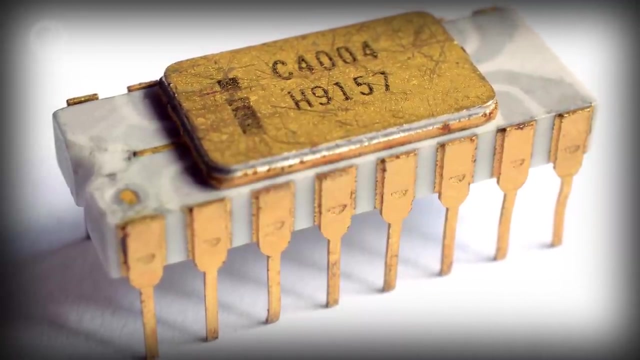 more complicated. Now. our example CPU and instruction set is hypothetical, designed to illustrate key working principles. So I want to leave you with a real CPU example. In 1971, Intel released the 4004 processor. It was the first CPU placed in a single chip and paved the path to the Intel processors.